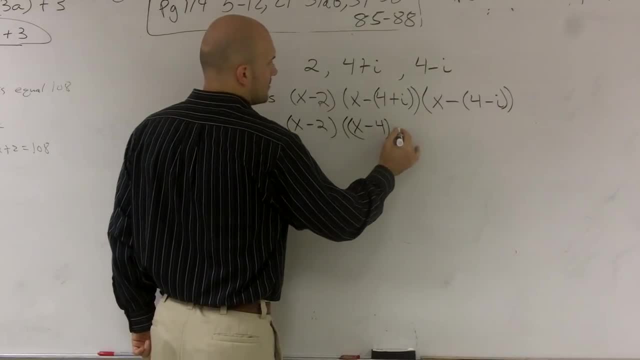 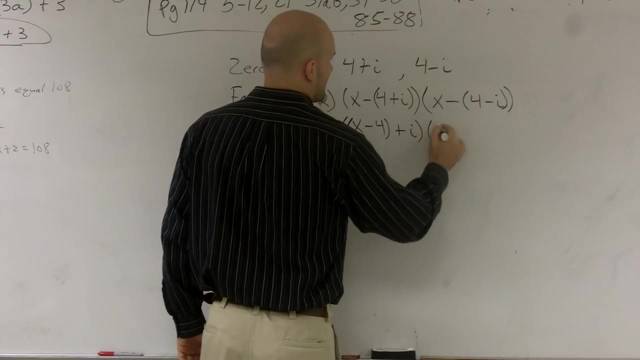 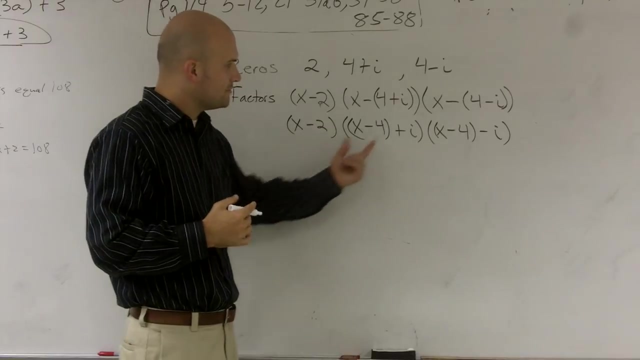 I'm going to group the x minus 4, let's see x minus 4 plus i and x minus 4 minus i. And the reason why I want to do this is because now, if you look at this, you're going to 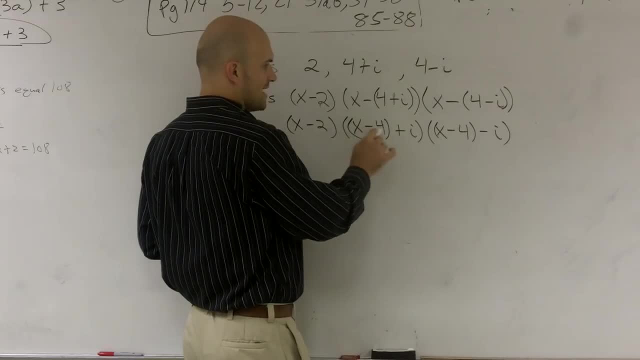 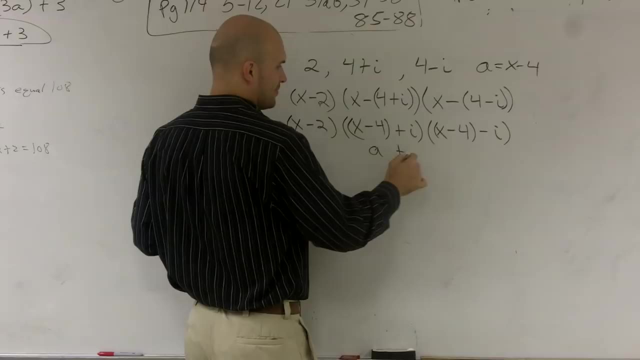 see that this is really kind of like an a. Let's pretend x minus 4 is a. a equals x minus 4.. So therefore it's a plus i times a minus i, And now what you know is we have a difference. 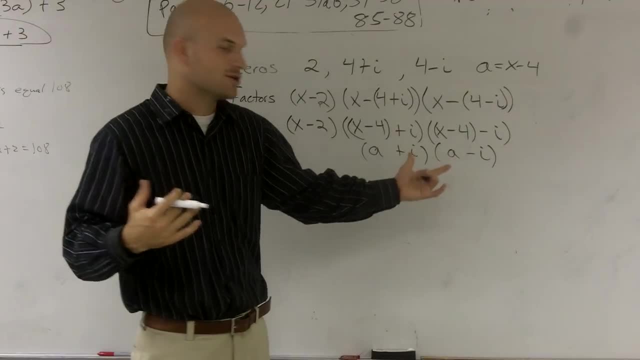 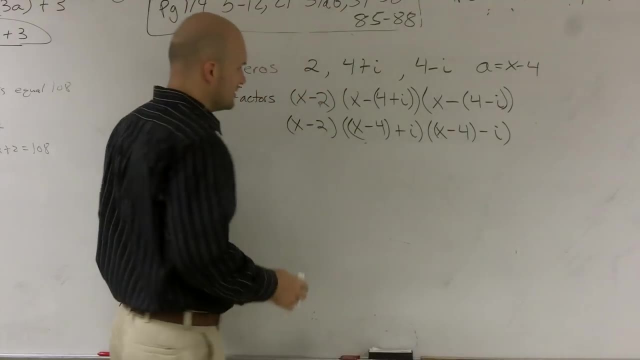 of two squares. So when I multiply these, I'm going to get rid of my middle terms. So this is something very important that you always want to look out for in mathematics. So what happens is, let's say, let's multiply these. So if I'm multiplying these by x minus, 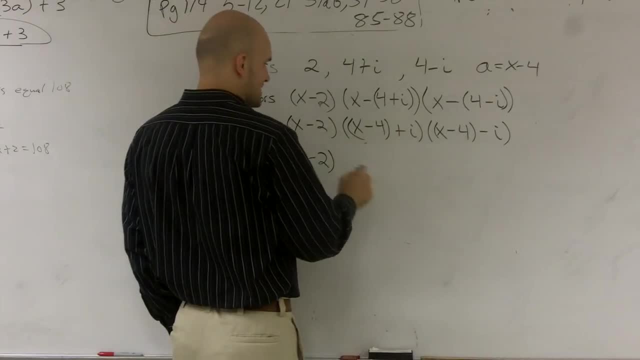 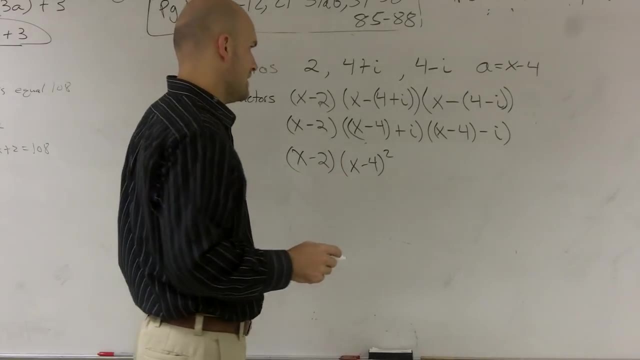 by these, so x minus 2.. So I have x minus 4 times x minus 4 is going to be x minus 4 squared. And then this is going to give me i times negative. i is going to give me a negative, i squared. 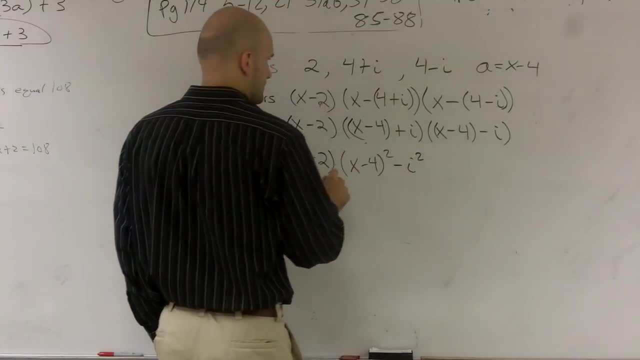 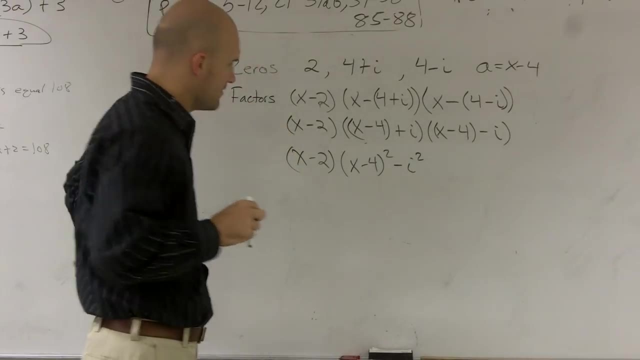 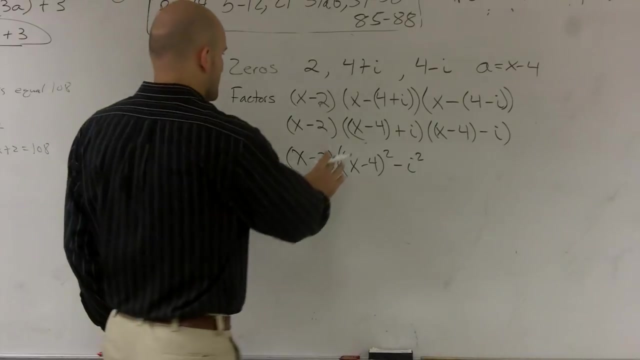 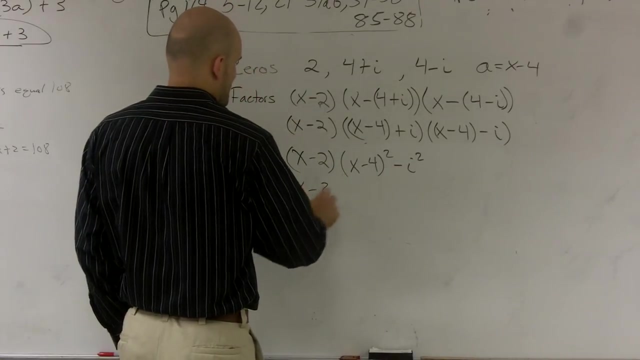 And then let's see if we get something. multiply these, Get my product here. i squared is going to give me negative 1.. So let's go ahead and figure out my x minus 2.. x minus 4 squared is going to give me x squared. 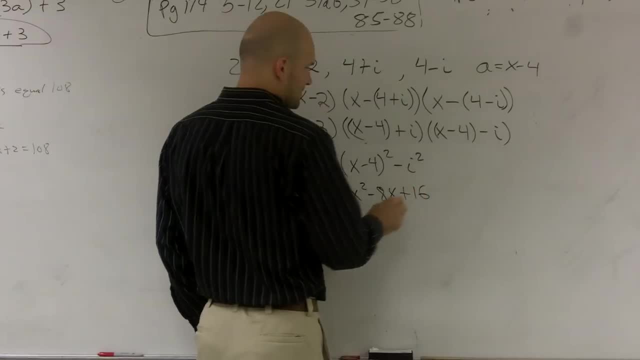 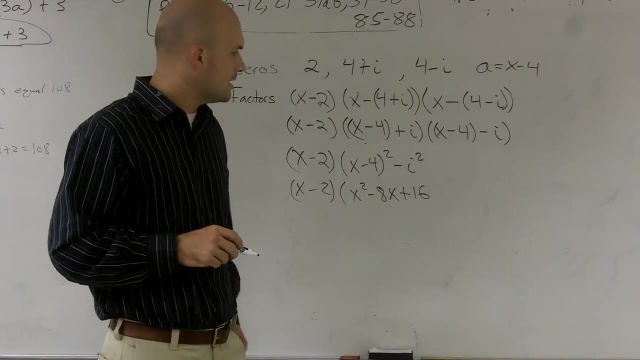 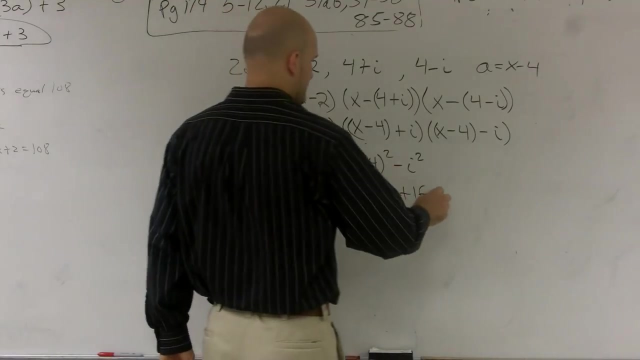 minus 8i, 8x plus 16.. And then here I have a. i squared minus 1 is going to give me a negative 1.. But times i squared is negative 1.. Negative 1 times this negative is going to give me a positive 1.. 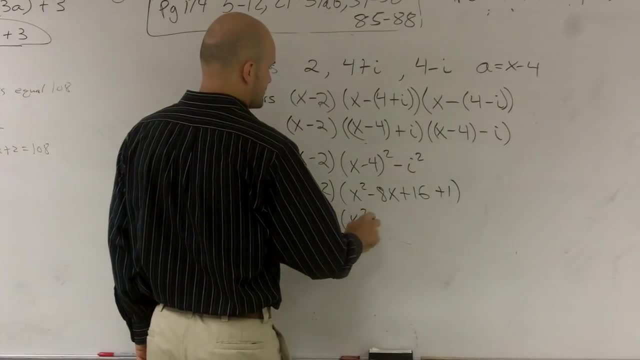 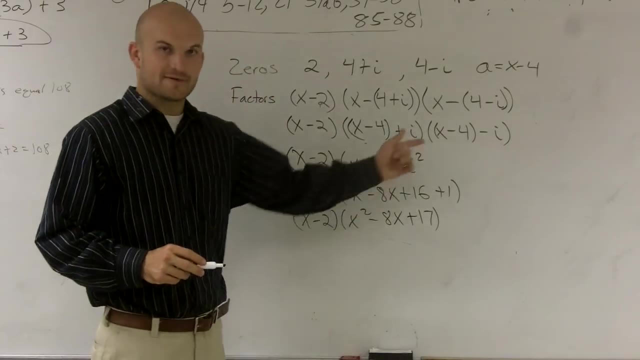 So therefore, I have x minus 2 times x, squared minus 8x plus 17.. Now I have to multiply my binomial times our trinomial, And again we're just going to use: make sure you multiply every term times, every term. 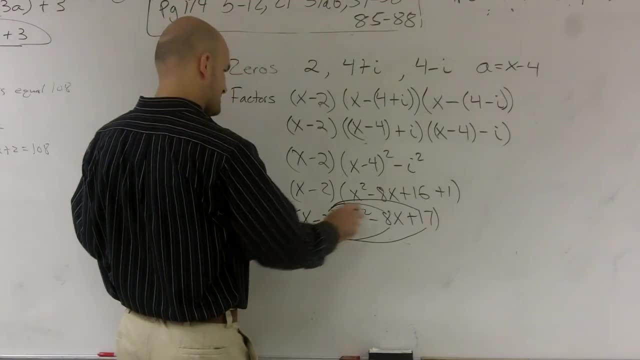 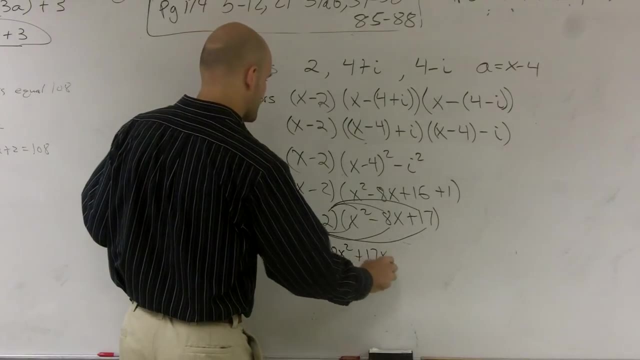 So let's see: x times x squared is x cubed. x times negative: 8x is negative. 8x squared x times 17 is going to give me a positive. 17x Negative. 2 times x squared is going to give me a negative. 2x squared. 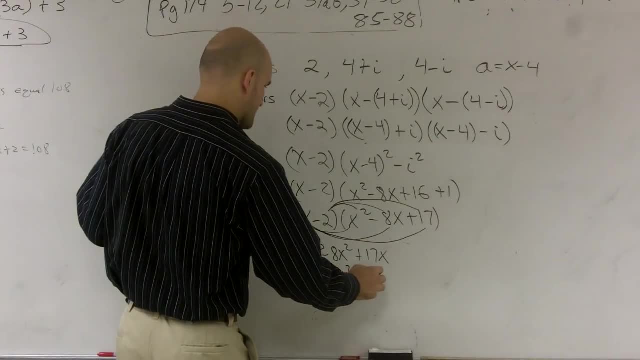 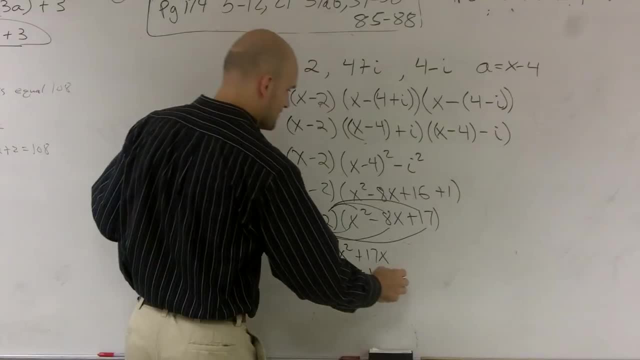 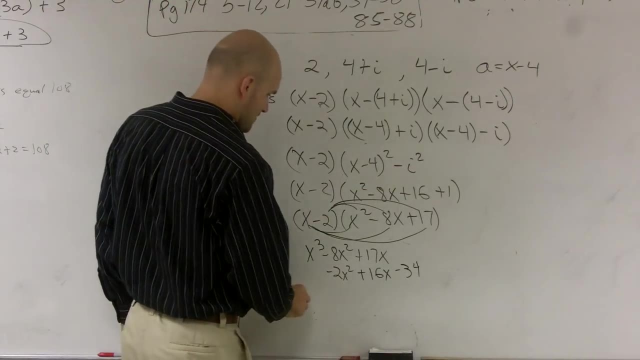 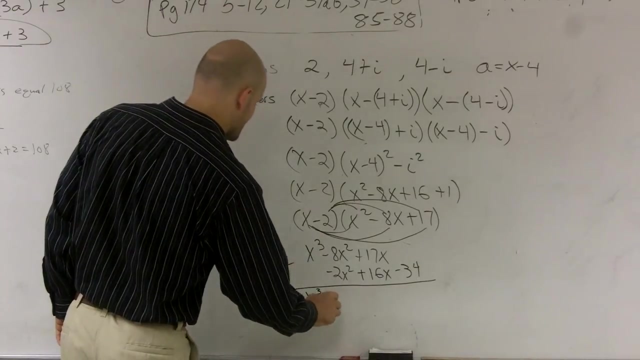 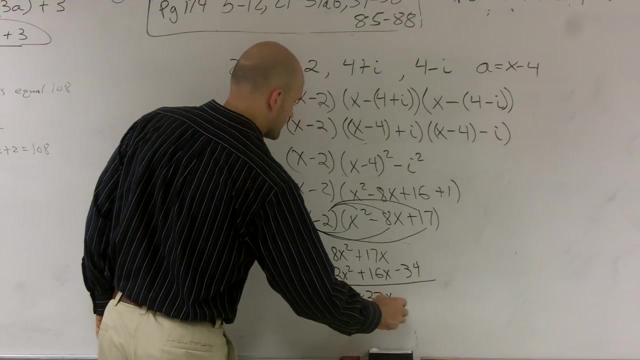 Negative 2 times negative. 8x is going to give me a positive 16x 16x and negative 2 times 17,. negative 2 times 17 give you negative 34, I can just combine these now to give me x cubed. let's see minus 10x squared. let's see plus 33x, minus 34.. 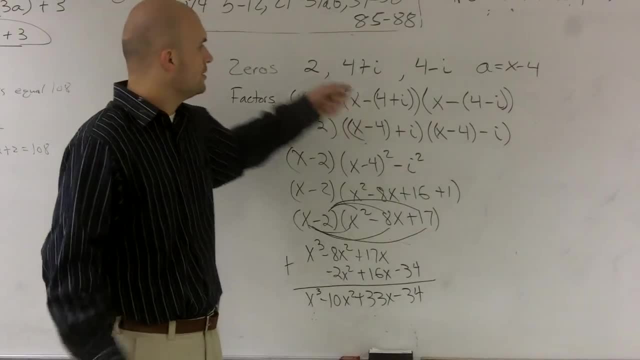 So that would be my third degree polynomial, given the zeros of 2,, 4 plus i and 4 minus i. 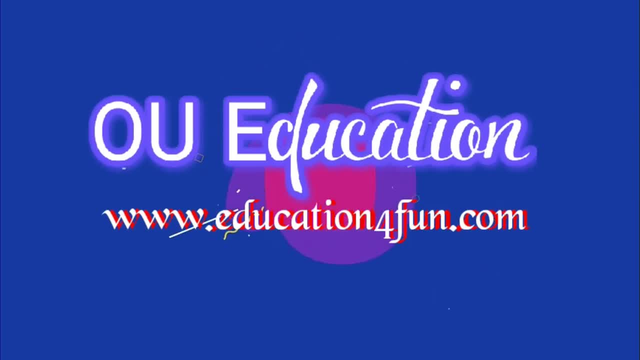 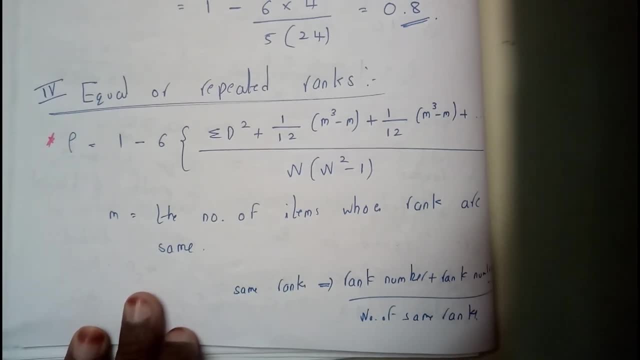 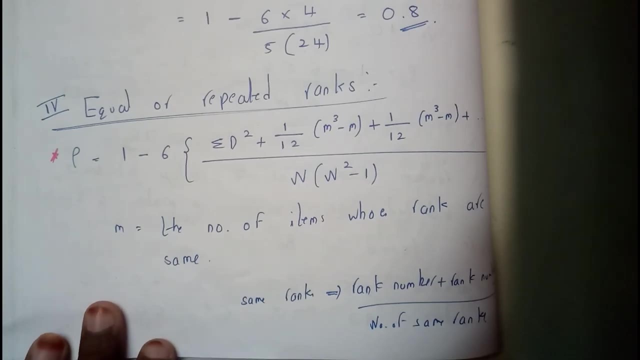 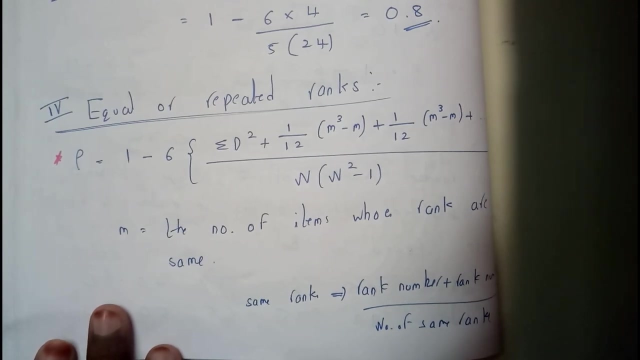 Hello guys, we are back with our next tutorial. In this tutorial we will be going through the second case, if there are any equal ranks or equal marks. So it is nothing. but rho is equal to 1 minus 6 into sigma d square plus 1 by 2 l into m cube minus m plus 1 by 2 l. 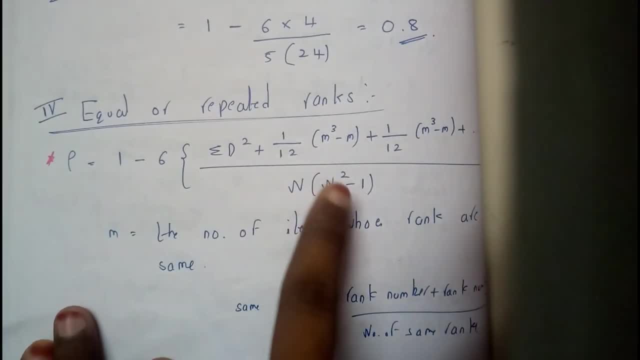 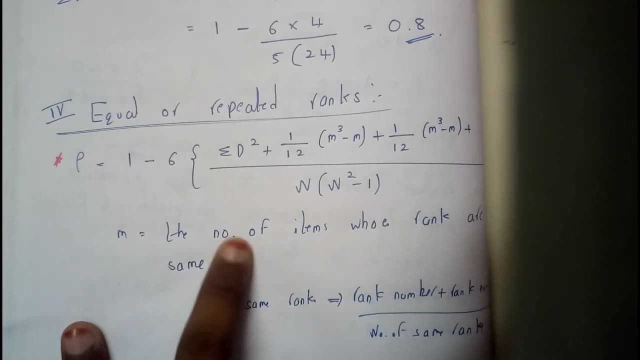 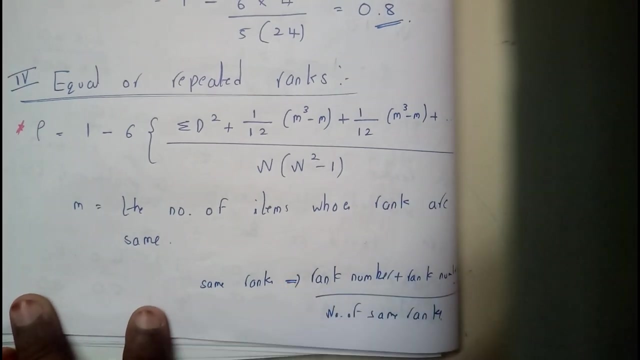 into m cube minus m, and so on up to infinity, by n into n square, n square minus 1.. So m is the number of items whose ranks are same. Same rank is equal to rank number plus rank number plus rank number by number of ranks. You will be understanding this formula once.